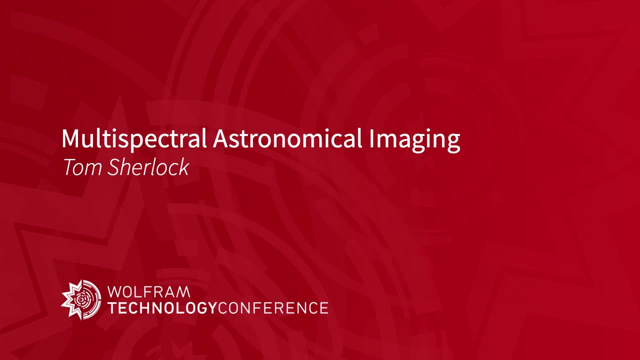 which is astronomy and astrophotography, And I try to do most of the work with Mathematica, And so today I'm going to be talking about automating an astronomical observation using Mathematica And a package that I've written, which is also available for download. So let's get started. 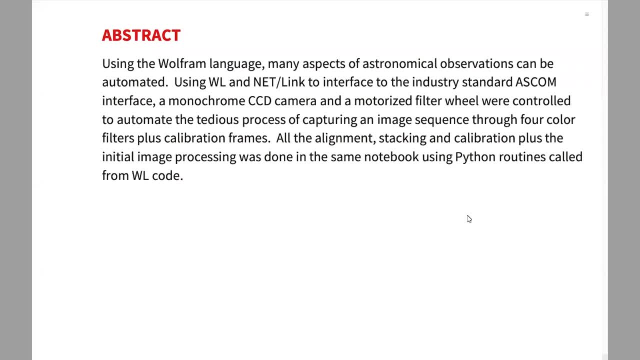 So I'm going to talk about doing traditional astrophotography with a monochrome CCD camera And I'm going to show the process that is used to collect the data for that and how you can automate that using the Wolfram language. And. 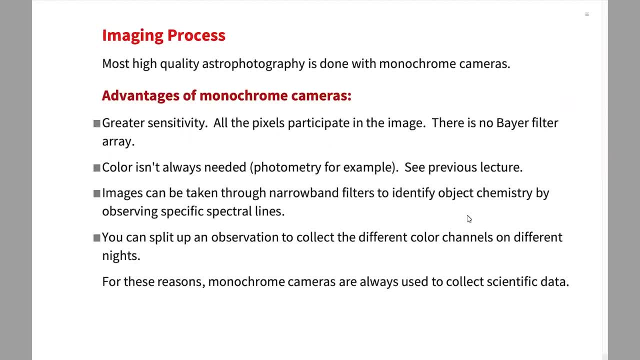 so let's see what we're getting into here. A lot of people think you know, when you do astrophotography, you just take a picture of the sky and you have something there. but it's not quite that simple And 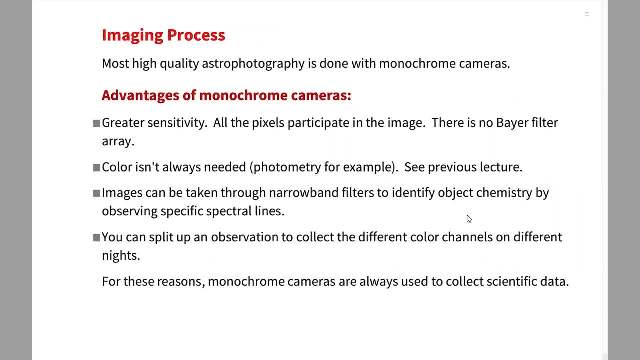 most quality astrophotography is done using what's called a monochrome camera, which only takes a black and white image. So you say, what is it? You know, you see all these great pictures coming from the James Webb Space Telescope or the Hubble Space Telescope. They're 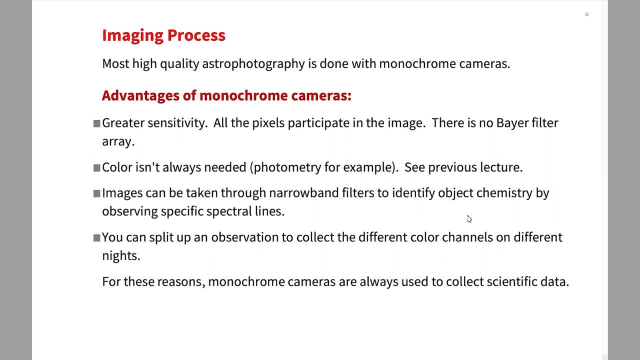 all in beautiful colors. Well, I got news for you. Those are all taken with black and white cameras. They're taken through a series of filters, And so there's advantages and disadvantages of that. We're going to go through some of the advantages and some of the disadvantages, and how. 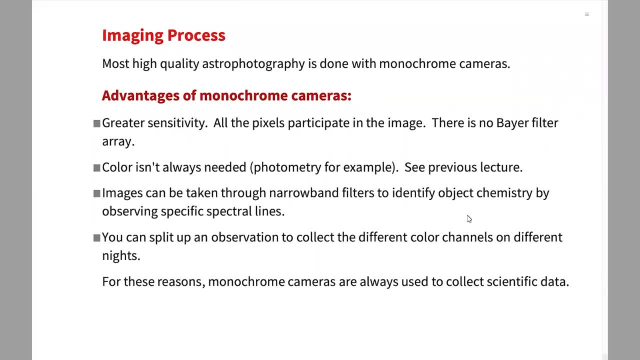 the Wolfram language can be used to speed things along and make things easier. Advantages of monochrome cameras is they're more sensitive, So all the pixels in the camera participate in the image. So what I'm talking about here is you say, well, you know. 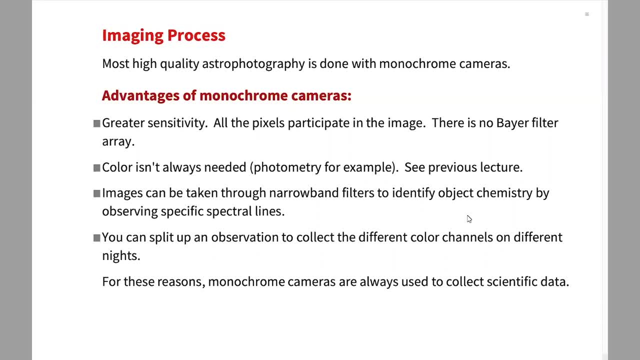 the camera in my iPhone is a color camera. Well, no, it's a monochrome camera. But what you don't realize is that in front of the CCD sensor in your iPhone, there's an array of filters, And there can be usually red, green and blue filters, or they can be cyan, magenta, yellow filters, but they're arrayed in like a checkerboard, And so you can see that there's a lot of different colors, And so you can see that there's a lot of different colors, And so you can see that there's a lot of different colors, And so just try to know where that is, And you can find it in the color. 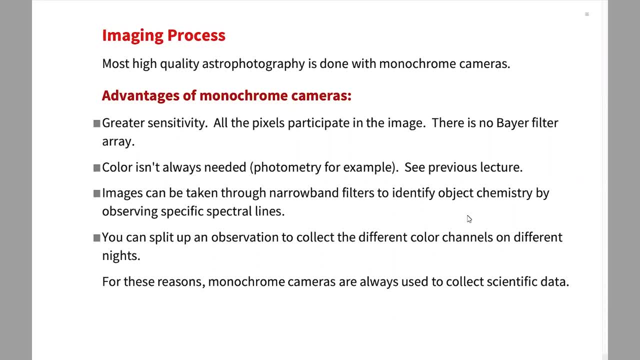 board pattern And the color picture that you get is: the process is derived mathematically from the signals coming from different chunks of that grid And it's interpolated through a process called de-mosaicing, And you can get astronomical cameras that do that, But the better quality. 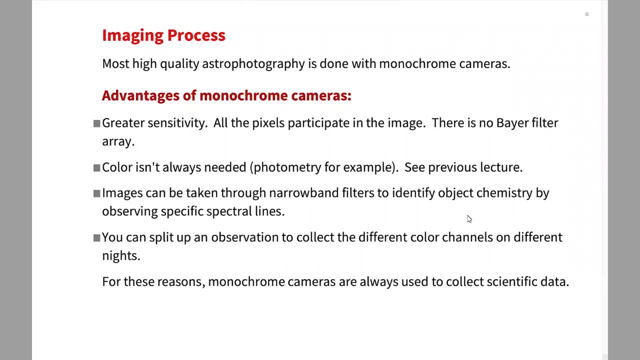 cameras, the better results are obtained with using a monochrome camera and putting separate filters across the sensor. So that's what we're going to going to talk about today, So you get greater sensitivity. Color isn't always needed. Sometimes you don't need or want color in your image, like to do photometry. I gave a lecture about this, a. 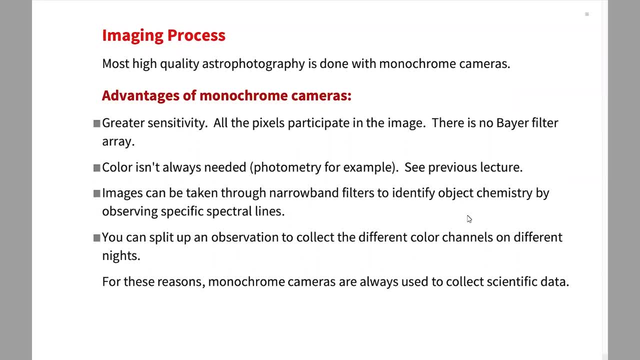 couple of years ago And you're really just interested in pixel electron counts then, So color isn't really necessary And you can do that with a monochrome camera. You can also extract scientific data, And this is the real reason why cameras like this are used on all space probes. 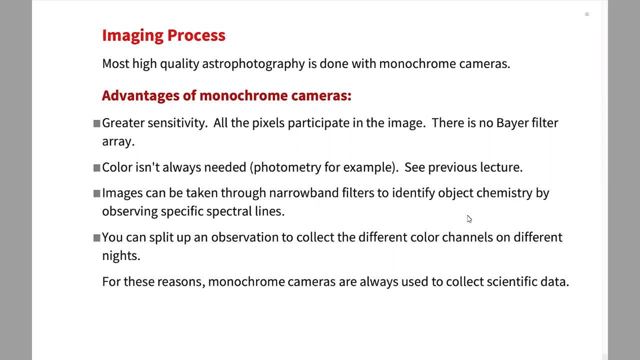 I think the latest rover that was sent to Mars. it was the first one that actually had actual color cameras on it. But the scientific cameras are still monochrome cameras. So you can use this to get scientific data through, for instance, narrow band filters to observe specific spectral. 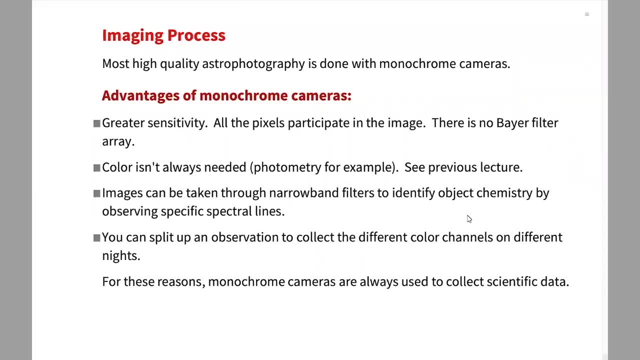 lines. And another thing you can do is you can split up an observation to collect different color data. It doesn't all have to be different colors. It doesn't have to be different colors. It can be done on the same night or at the same time. It can be done across a series of weeks or 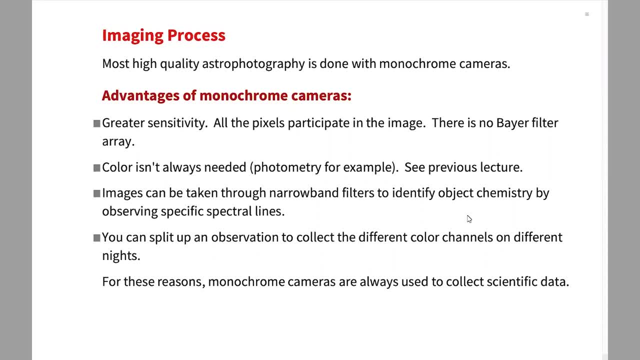 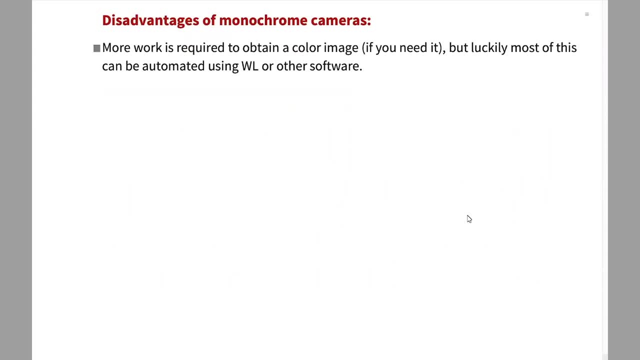 months, And you can just assemble everything when you're done So for these reasons, monochrome cameras are always used to collect scientific data. Disadvantages: it takes more work to obtain a color image if you need it, But luckily you can automate most of this stuff using Wolfram language. 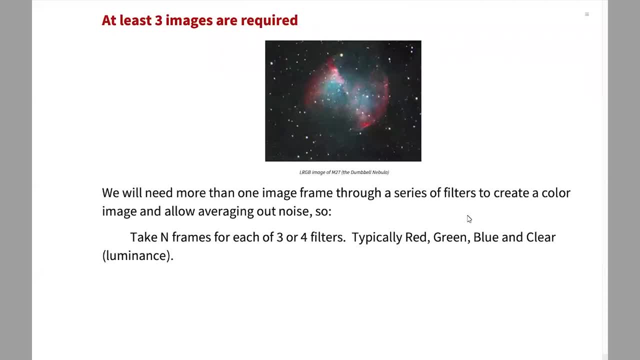 or other software, But we're going to use Wolfram language. So to get a color image like this- this is a picture of M27. The Dumbbell Nebula- You need at least three images: one through a red filter, a green filter. 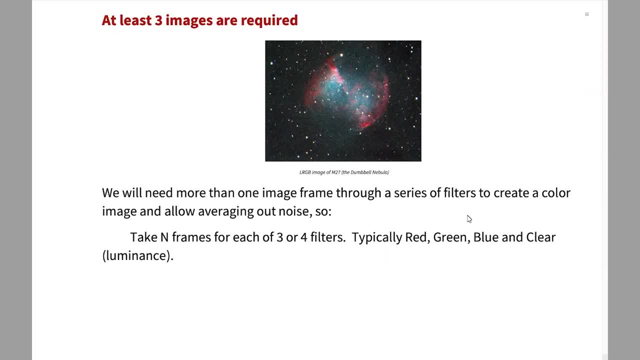 and a blue filter. Typically it's done. you do it with four images. You take three color images and then a black and white, what's called a luminance image, through just a clear filter And you combine all four of them And the luminance image will enhance the spatial. 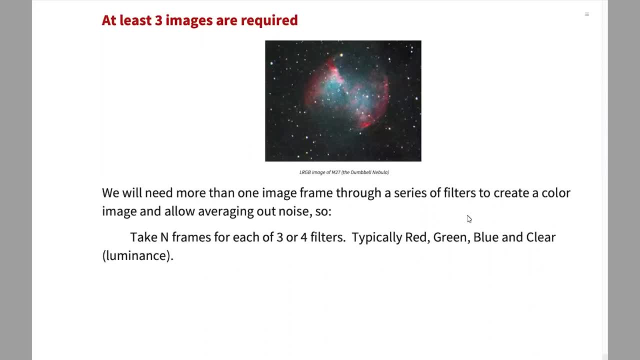 data in the image And the color data will just do the color image. Is that black and white instead of monochrome? Is that grayscale or is it pure black and white? It's grayscale. I'm just using these terms loosely: black and white. 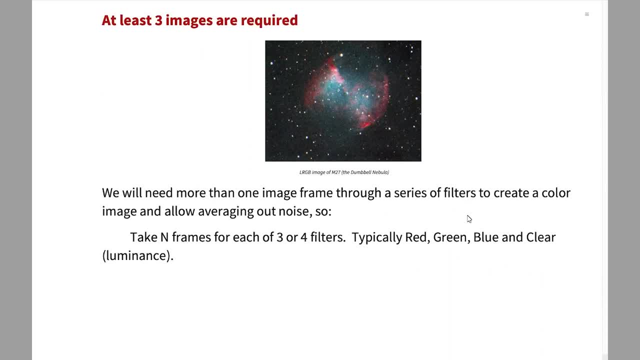 By monochrome I mean a grayscale camera. Okay, So unfortunately, in order to minimize the noise with astronomical image imaging, you need to take more than one image and you combine them to average out the noise. So for each one of the filters you're going to be taking a sequence. 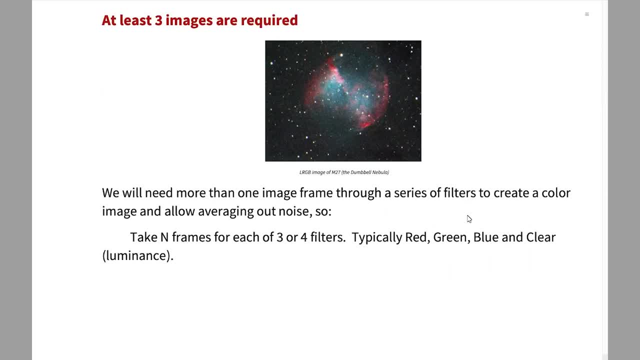 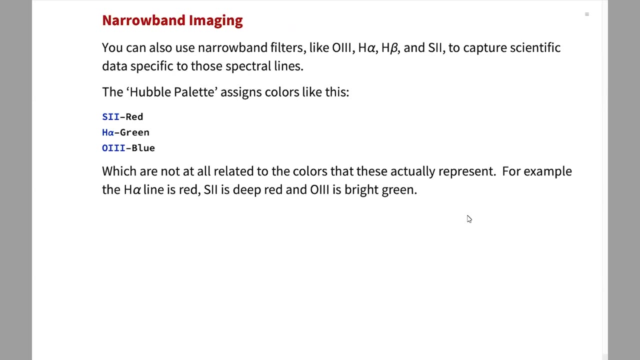 of images And since you're taking it through possibly four filters, you're going to be taking that sequence four times And you can also use narrowband filters. These are specific filters that isolate different parts of the spectrum, For instance, sulfur, two transition, the hydrogen alpha lines or oxygen three lines. 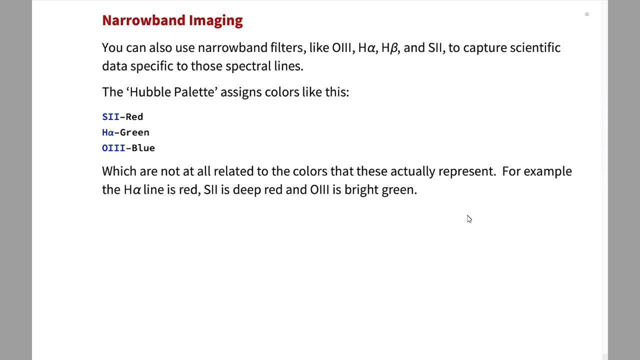 And you can use this to determine the distribution of different elements in an object that you're looking at. A lot of nebula glow strongly in oxygen three light And you can see that by assigning a color to the light coming from the oxygen three filter. 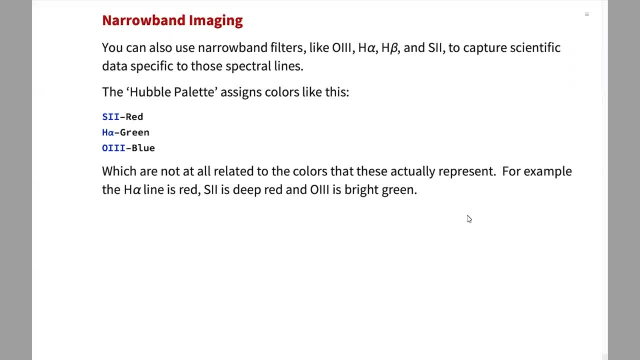 And there's actually something called the Hubble palette, which is kind of a standard palette used by the Hubble Space Telescope, And this assigns the sulfur two line to red, hydrogen alpha to green and oxygen three to blue, And which is a bit of a fib because those lines are 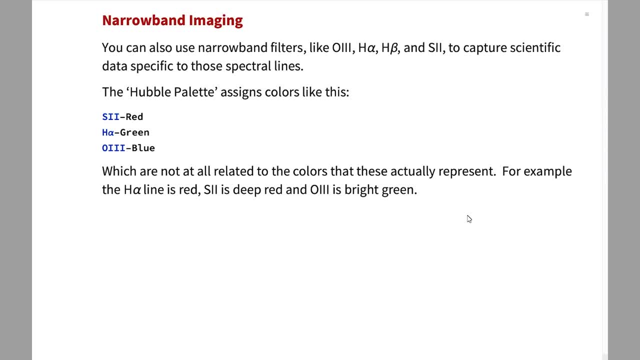 nowhere near those actual colors. For instance, hydrogen alpha is bright red, Sulfur two is a deep red And oxygen three is a bright green, But here we're calling it blue. But you can do that to create a false color image, And the purpose of that image is not necessarily to show what the thing 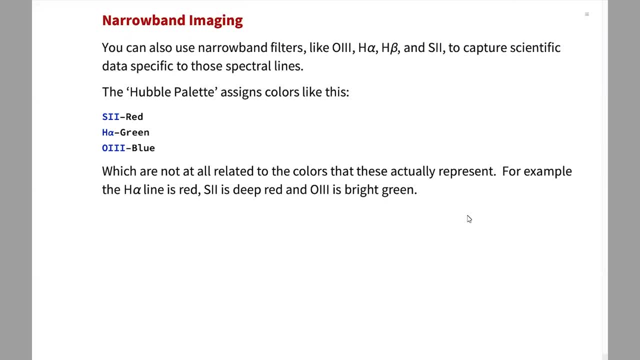 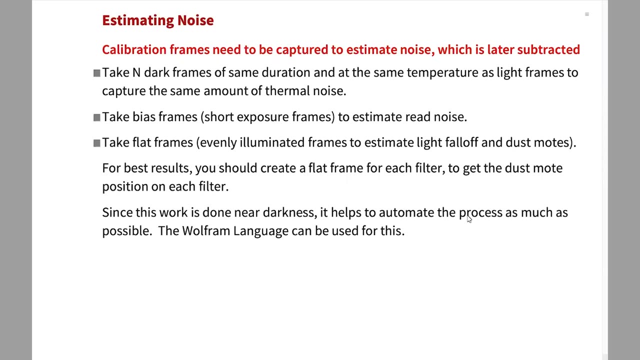 would look like out in space, but to show you where the light is, And so you can see that the elements are distributed in that image. So that's why this type of imaging is done, for scientific work. So, as I said before, we have to- and I've said this before and I've done all sorts of 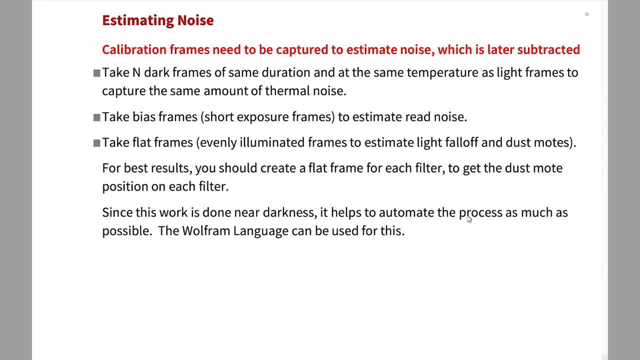 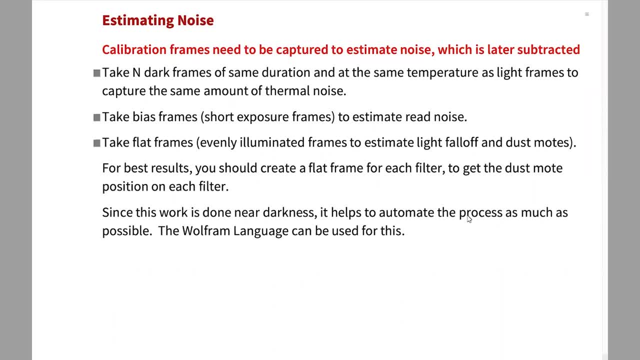 signal-to-noise ratio. So the way we do this is we take a lot of images, we align them and average them out and that will average out the noise and enhance the signal. So there's different types of noise. There's thermal noise, There's readout noise And then there's like geometric noise. 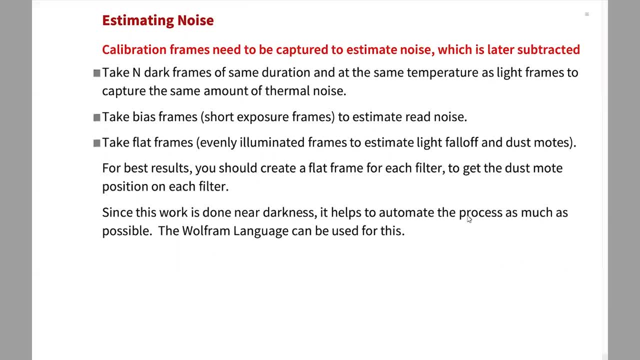 And we take a series of what are called calibration frames to eliminate each one of these effects. And when you're doing multispectral imaging, it has the additional complication that you have to take the flat frames which for each filter, because each filter probably has different particles of 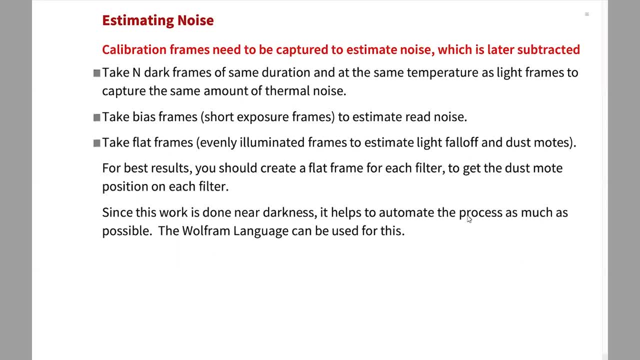 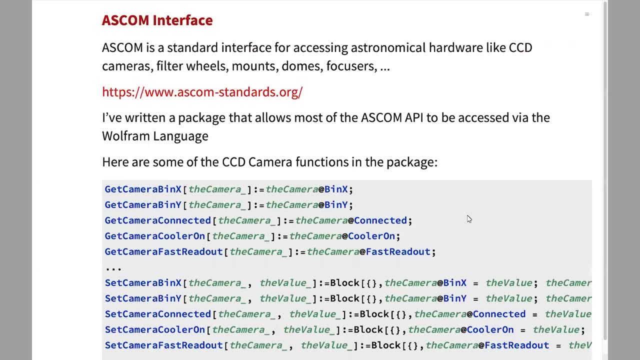 dust on it And they produce donuts in the image. So you really have to calibrate each one of those filters, But we can do this easily using the Wolfram language. So the way I did this is using the standard image And I'm going to show you how I did it. So I'm going to show you how I did it. 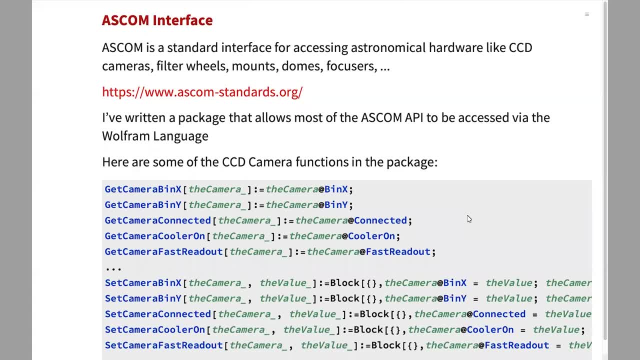 So I'm going to show you how I did it. So I'm going to show you how I did it. And this is an API described in ASCOMstandardsorg, which is used to access all sorts of astronomical instruments, For instance cameras, focusers, filter wheels, domes, the telescope mount. 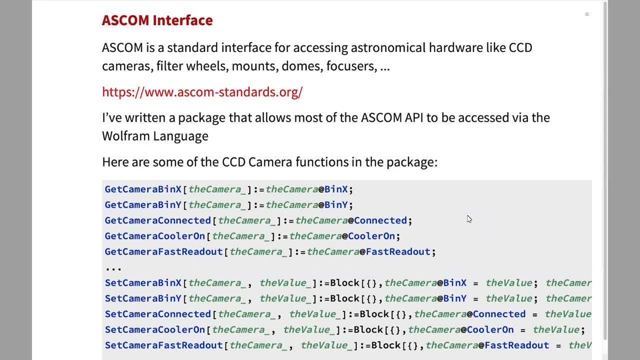 rotators, a bunch of different things. Chances are they have an ASCOM set of drivers written for them And I'm going to show you how I did it. So I'm going to show you how I did it And this is an. 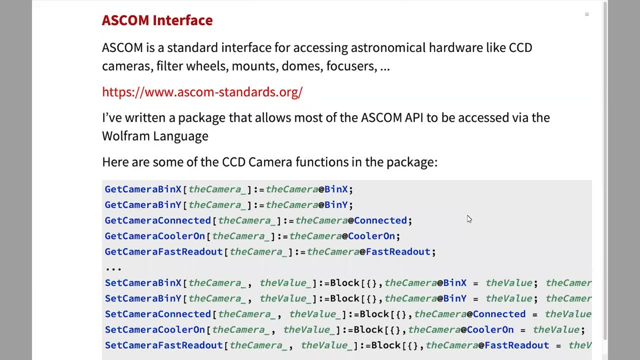 Almost, if not all, the ASCOM API. I've wrapped in a package which I call astrodevicem, which is part of the downloads for this lecture And that will let you use the Wolfer language to talk to the ASCOM API. 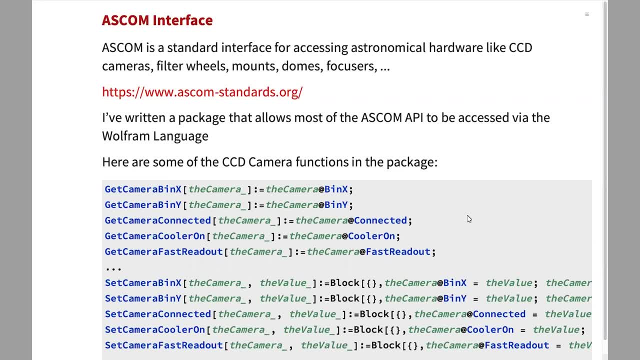 And this is a little chunk of astrodevicem. So, for instance, here you can see that I'm getting the camera's binning factor, whether the camera's connected. So these are some get and set methods. So, given the camera, it'll tell you what the binning is, whether it's connected. 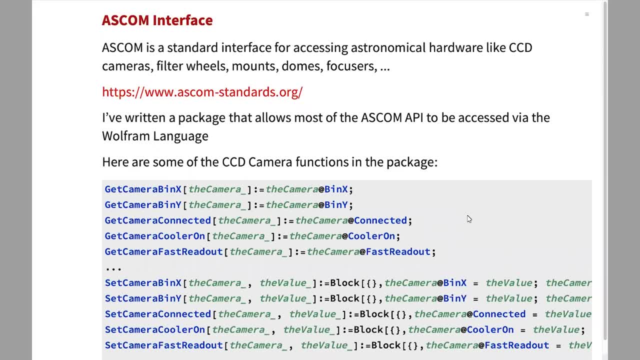 whether the thermoelectric cooler is on, whether it's capable of fast readout, and you can set the stuff too. So this is just a little chunk of a large file. There's a problem with astrodevicem? It may be a problem. it may be not a problem. 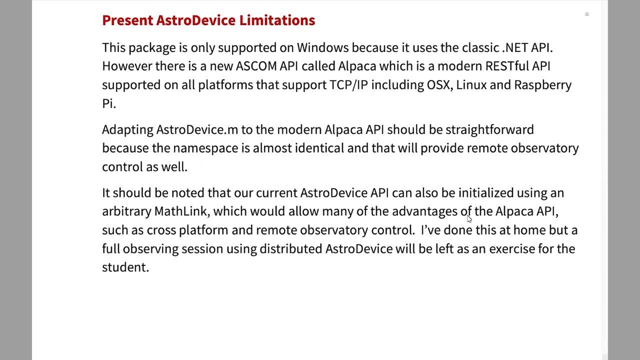 Right now, this package uses Netlink, which is a Windows-only API, So that's a limitation if you're working on Mac or Linux. However, there's good news. The ASCOM standards are building a new API called the Alpaca API, which is a RESTful API. 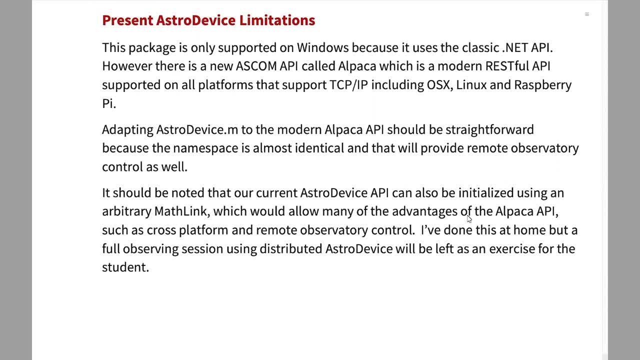 It only requires the ability to have TCP on your system. So it's supported on all platforms. And luckily the namespace for the Alpaca API is virtually identical to the classic ASCOM. So in the next month or two I will roll out a new version of Astrodevice which will 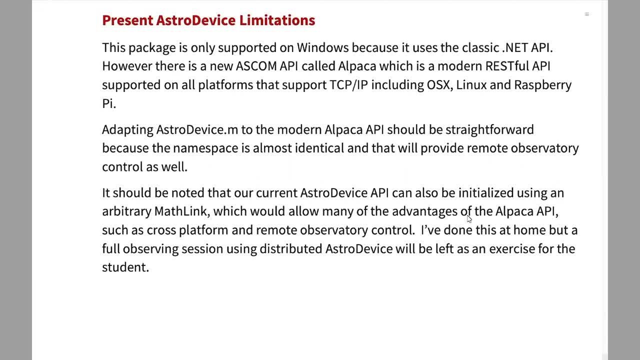 talk to the Alpaca API, But for the inpatient, I should note that the Netlink interoperability layer in Mathematica can also be initialized using the regular Mathlink. So you can basically get most of the advantages of Alpaca right now, today, by just using the. 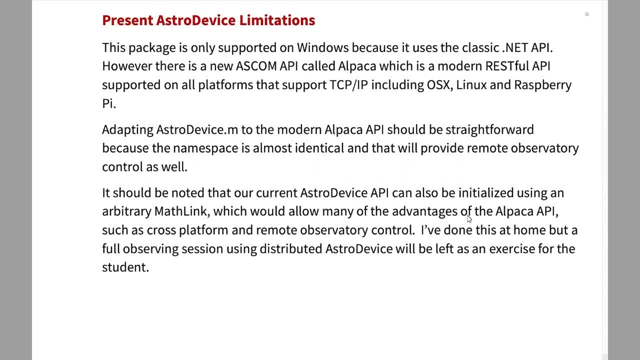 Mathlink, and then you can have two different computers, Which don't have to be in the same room, but you can be in different parts of the world talking to each other. You can do all this stuff on your Macintosh and have a Windows machine connected to your. 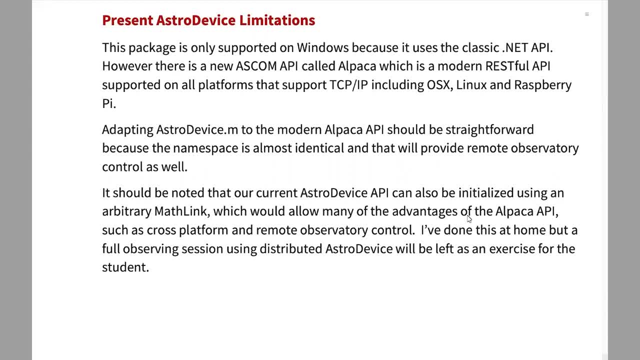 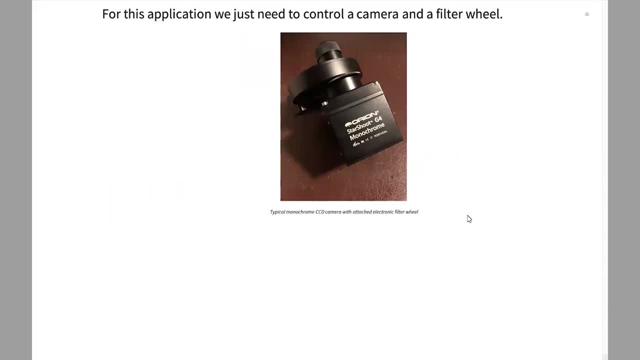 telescope and your camera. But that will be whether you want to try that. I've demonstrated that kind of in principle in my home, but the full application will be done by you. So this is the camera I use. This is a. 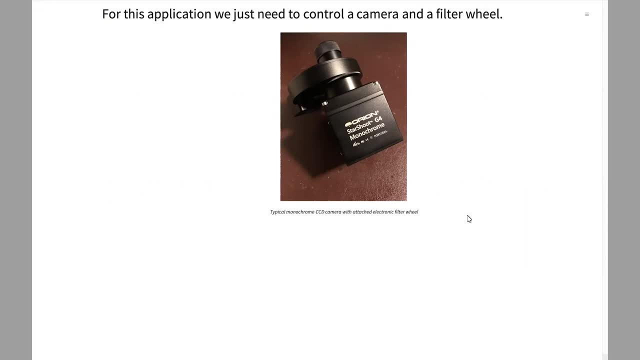 Very low-end monochrome imaging camera and the device on the front of it is the filter wheel, which contains five filters: There's red, green, blue, clear for luminance and an opaque one which is a substitute shutter for this cheap camera, which doesn't actually have a shutter built into it. 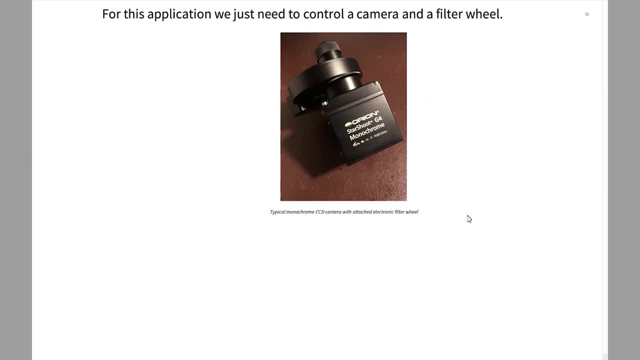 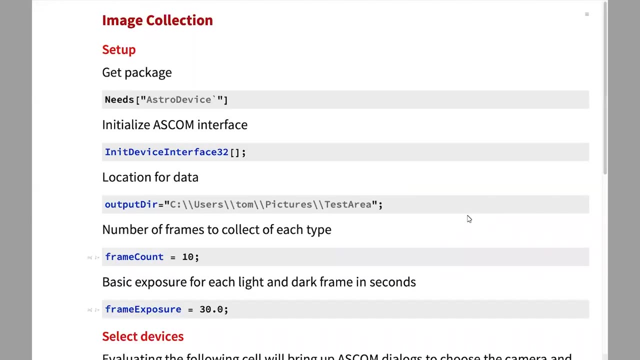 If I didn't have that, I had to put a hat over the end of the telescope. So it's a step up from the hat method, but it's not. It's not perfect, So let's see how we actually do this. 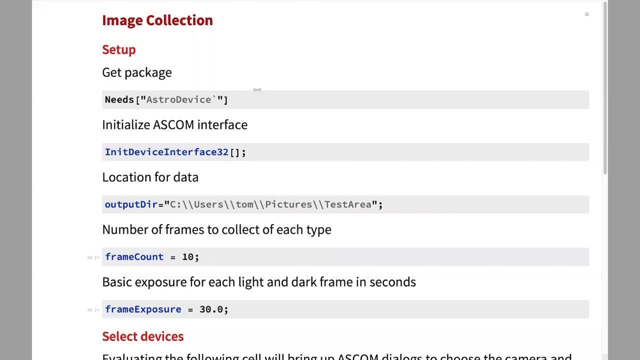 You do load. in the AstroDevice package, You initialize the interface- It's InitDeviceInterface32, because Ascom is currently 32 bits. You set up a data collection area, So the number of frames that you want to collect of each type. 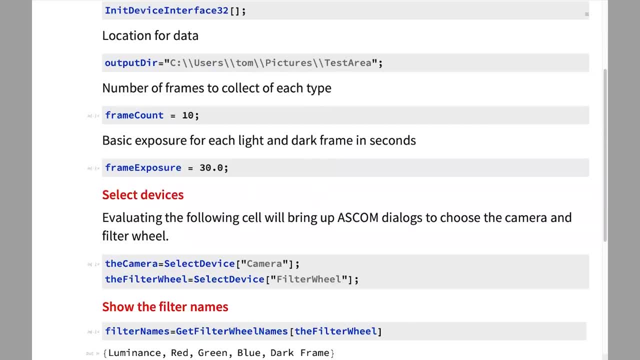 And the exposure. And then you have to. You have to get a camera device and for this example we're just using camera and filters. So we just need to get the camera device and the filter wheel device. And if you call these functions SelectDeviceCamera or SelectDeviceFilter, Ascom will throw up. 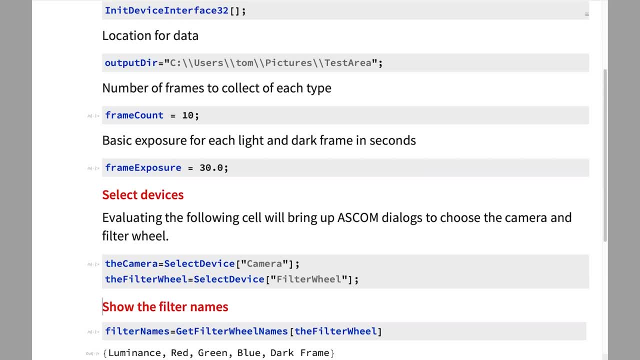 a dialogue box asking you to select which camera, because you may have several cameras on your computer or several filter wheels And one of the properties I set for the filter wheels. I gave actual names to the different filters, So I called them luminance, red, green, blue and dark frame. 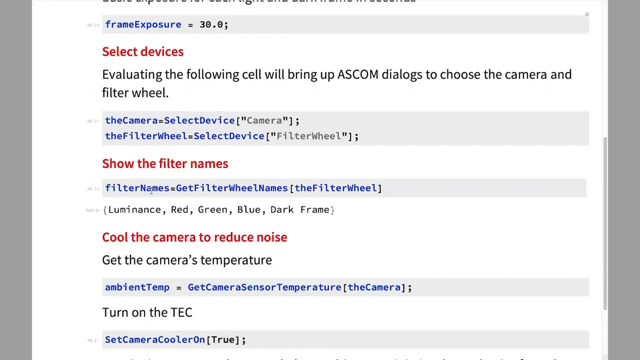 So then, if you call getFilterWheelNames, it will give you these easy-to-remember names And then we can start playing around with the camera. We can get what temperature the camera is at, So that'll tell you what temperature the camera is currently at. 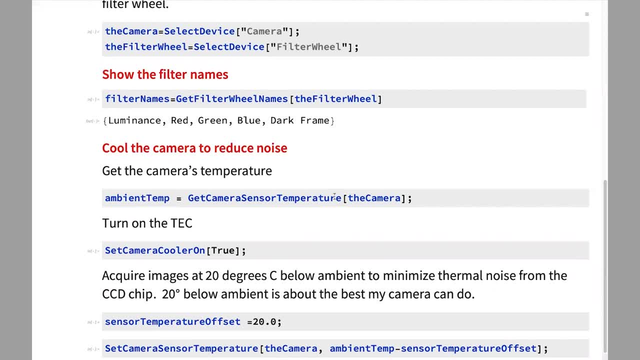 Then you can turn on the little refrigerator which is connected to the CCD chip, The thermoelectric cooler, And then you can set the camera to be 20 degrees below ambient. so set camera sensor temperature And that will start cooling the camera down. 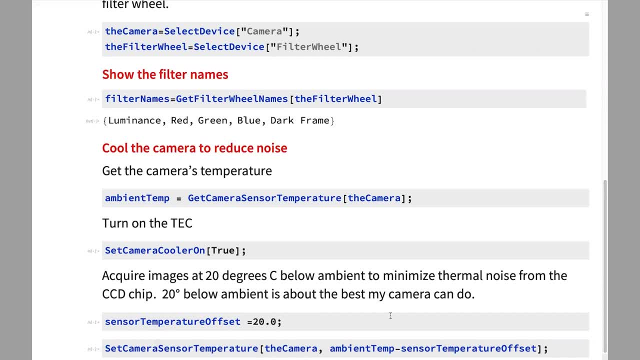 And this is important for another reason, because, since things like dark frames are dependent on the temperature, if you can always set the camera at a given temperature, then you can build up a dark frame library at a given temperature And then you can just use that. 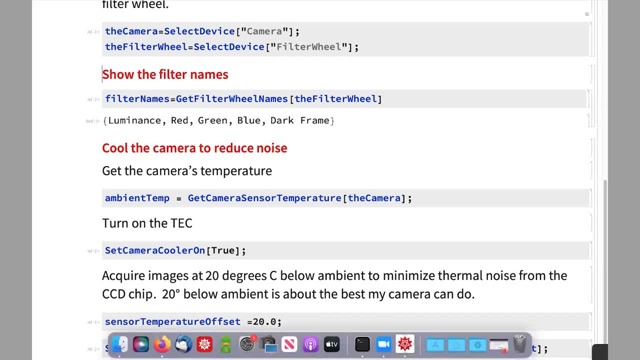 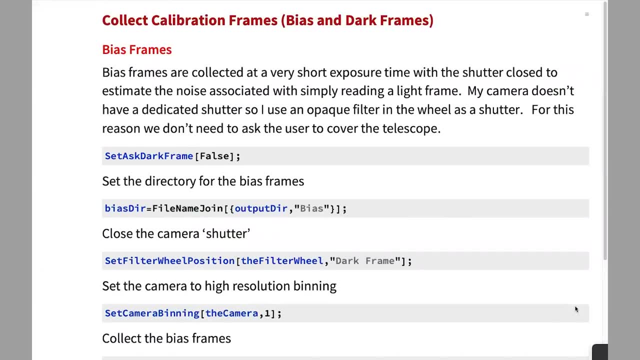 You don't have to recollect dark and bias data. So then we can – and, by the way, you don't have to do the calibration frames first. You can do this some other time, And if you have the library, you're good to go. 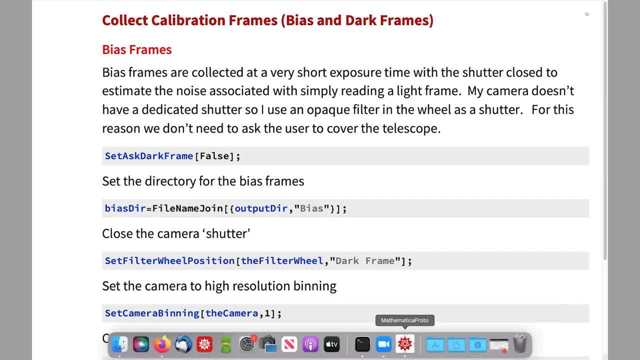 But this is how you would collect, for instance, a set of bias frames. Bias frames are – they just measure the noise that's associated with reading out data from the CCD chip, So it really needs – very, very short exposure. So this ass dark frame just – so mathematically it doesn't throw up a dialog box saying put: 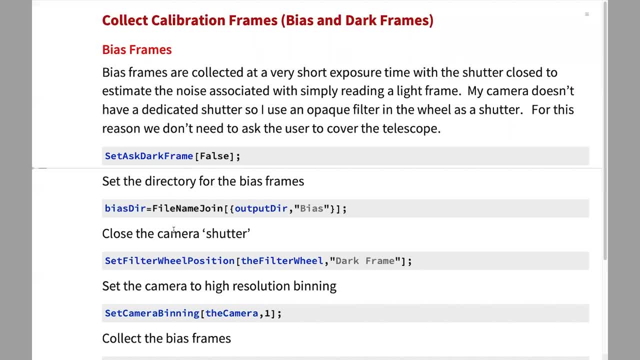 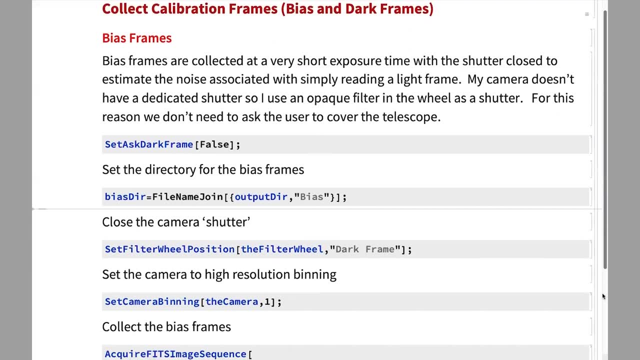 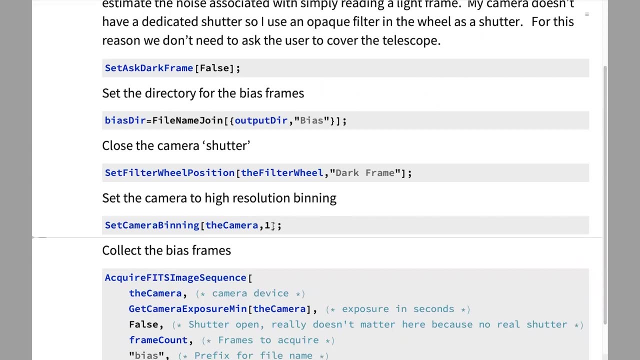 a hat on the telescope And then, since I've got a shutter on the camera, so I set up a directory for the bias frames, I set my filter wheel position to dark frame so that closes it off. I want to take high-resolution images, so I'm setting the camera binning to 1, so that's. 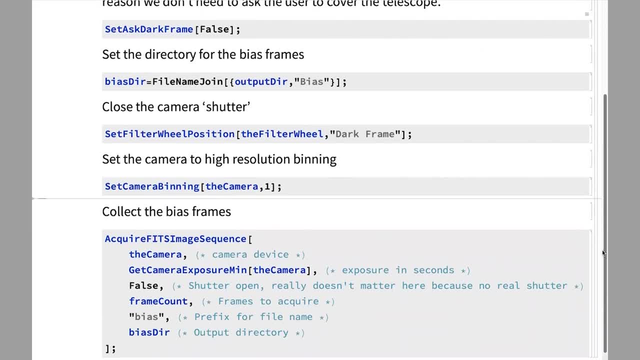 all pixels are individual pixels, and then I call this function acquire fits image sequence. So what this will do is this will take a sequence of images- frame count images- and store them in a sequence of fits files in my bias directory, and each one will have 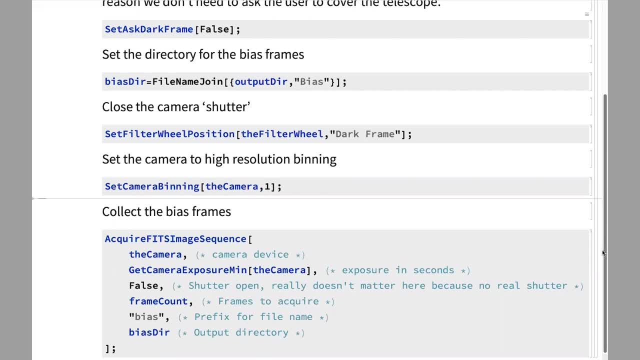 the word bias prepended to it, so I know which ones they are, And the false is just – you can also have this open and close the shutter on the camera, but since my camera doesn't have a shutter, it doesn't matter. 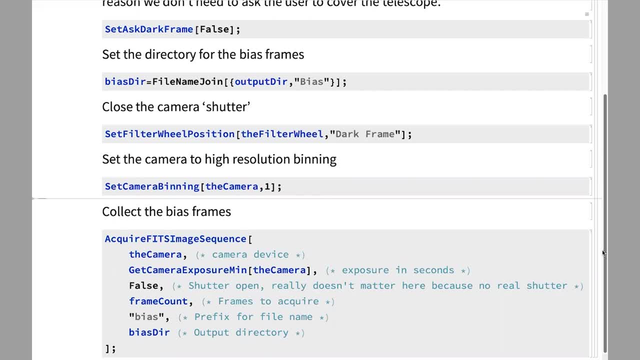 And also this particular thing: get camera exposure min for the camera. that calls the Ascom API to ask the camera what is the shortest exposure, because that's what we need in order to get just bias data. So that's what that is. 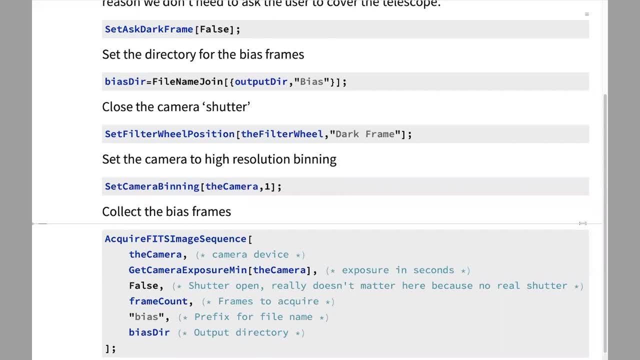 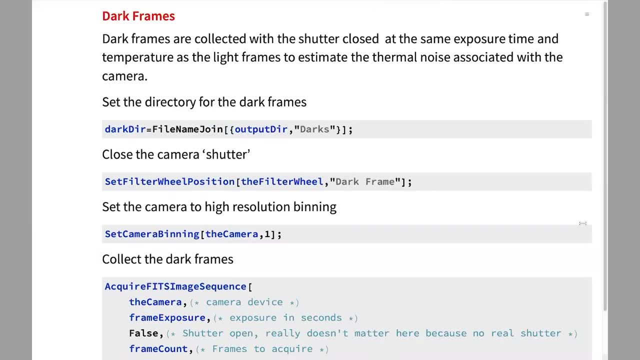 And then this will just process through it and take a sequence of things and you wind up with a series- It's a series of fits files in your directory. Same thing for dark frames, since the dark frames are just basically the same as bias. 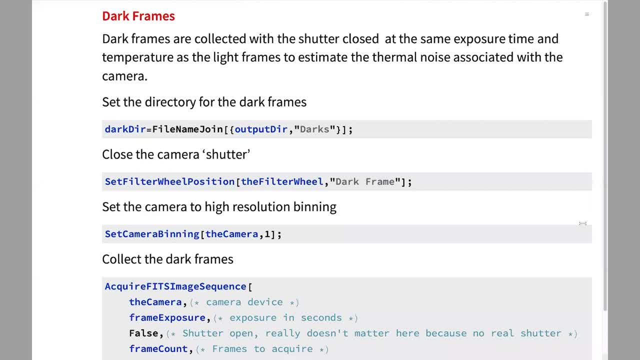 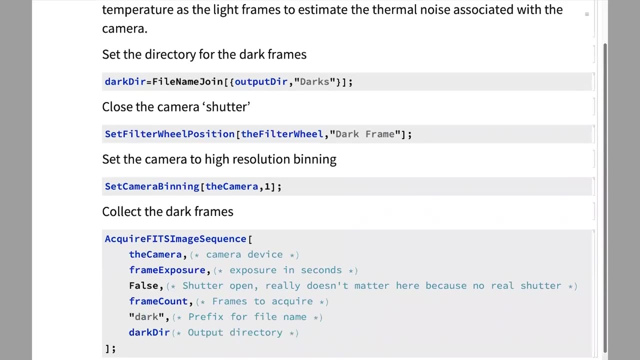 frames, except they're at the actual temperature and length of exposure that you're going to be using. It's the same exact thing, except that I store them in a different directory. I still have it set to dark frame, still dark, still setting the camera binning and it acquires. 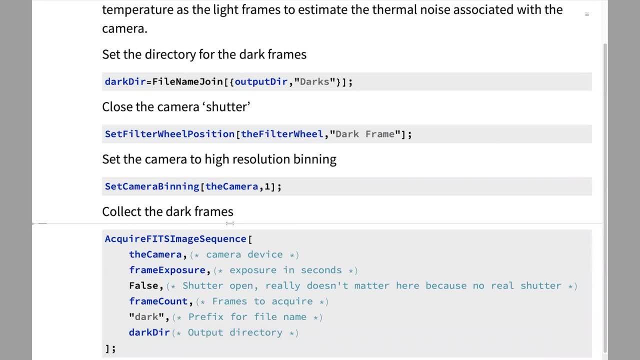 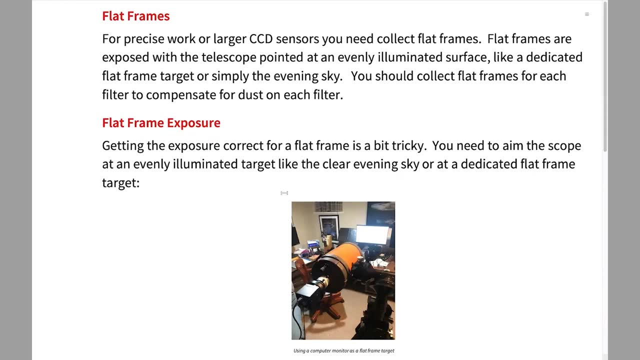 another fits image sequence. Now for flat frames. it's a little trickier because you have to. a flat frame is an image of an evenly illuminated object And traditionally the evenly illuminated object is like the twilight sky or the pre-dawn. 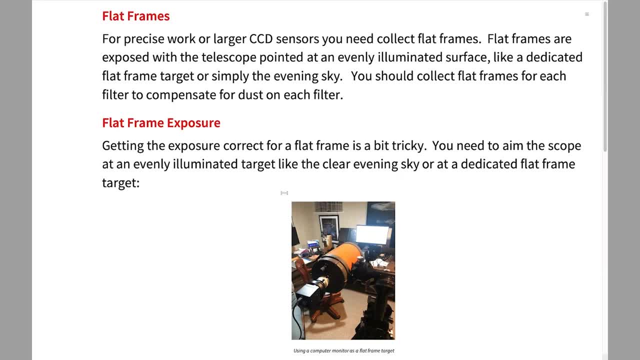 sky if you've been up all night. Or You can also aim the telescope at an evenly illuminated surface, for instance, like that monitor there which is in my basement office. So that's. These are all good ways to get flat frames. 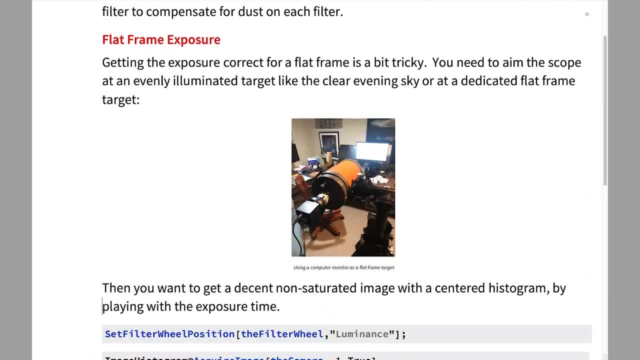 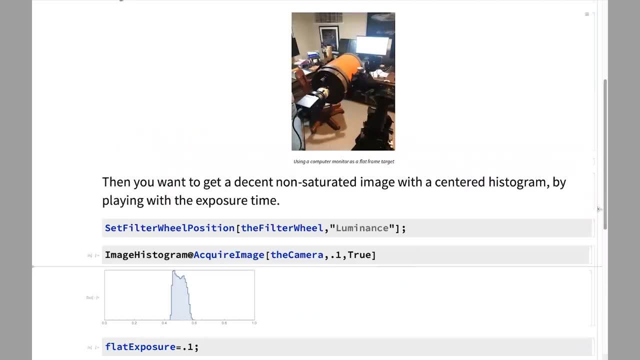 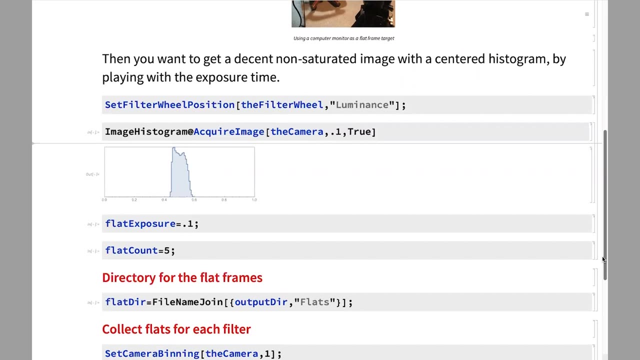 And But it's a little bit trickier than that, because you want to get a good exposure for the flat frames, And The way you can do this Is you want to get something that's not saturated, And it's easy to saturate the camera when you're pointing it at something like that. 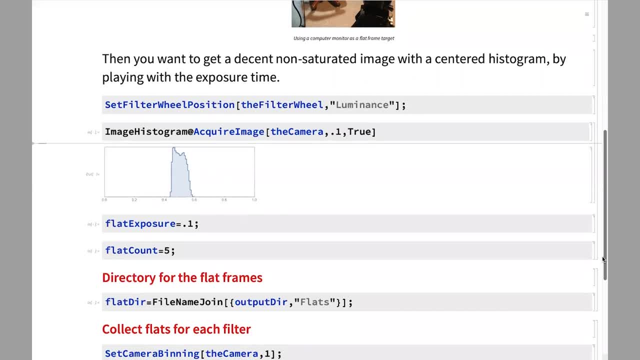 monitor or the evening sky. So you need to play around with the exposure And obviously the exposure is going to be different for whatever camera you have, until you get a histogram- And Mathematica makes really nice histograms- So that will be a histogram of a single frame brought off the camera of 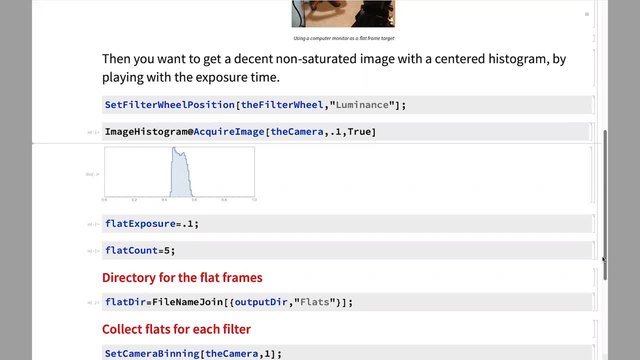 For a 0.1. 0.1., 0.1. 0.1. Second exposure. So that's what you want. You want something kind of in the middle like that. So we use that And if you think about it for a second, you should really do a separate exposure for each. 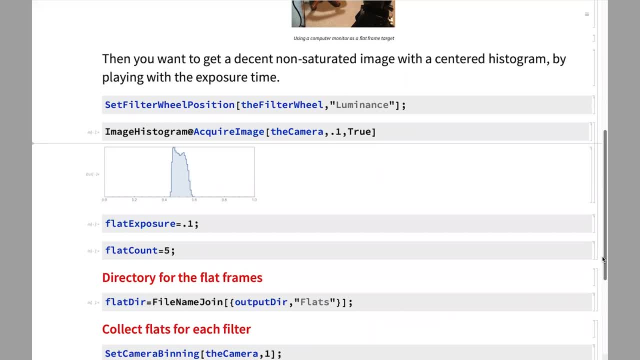 one of the filters, because they're going to have a little different response, So I'm glossing over that, but that's kind of what you need to do. So if we take five flats at 0.1 seconds, you set up your directory for the flat frame. 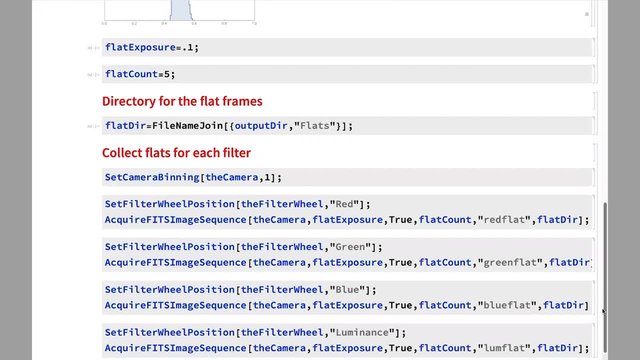 And then you collect flats for each filter And then you set up your directory for the flat frame And this sort of thing really beats screwing filters on for each one and resetting the camera and all sorts of nightmarish stuff that you don't want to do in pitch darkness. 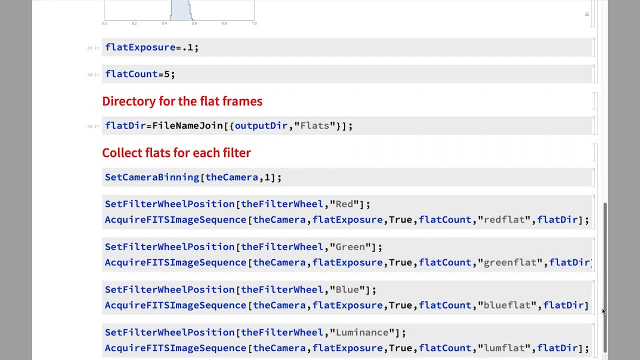 when you're dealing with cold and stuff. So this will just munch through all the different filters in the filter wheel and it will take a sequence of flat frames which will record positions of all the dust motes on your filters And store them in the directories we've set up. 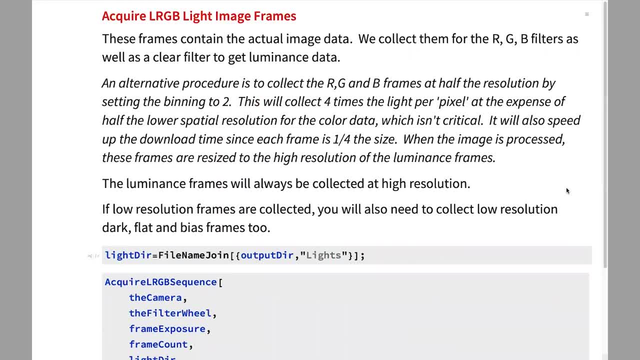 So that will get you your flats. And then we get around to acquiring the actual image frames. So this is where we actually take a picture of something in the sky. So the rest was just kind of the preliminaries, So for this. 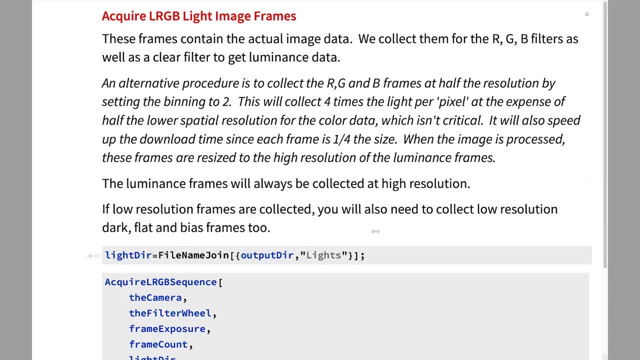 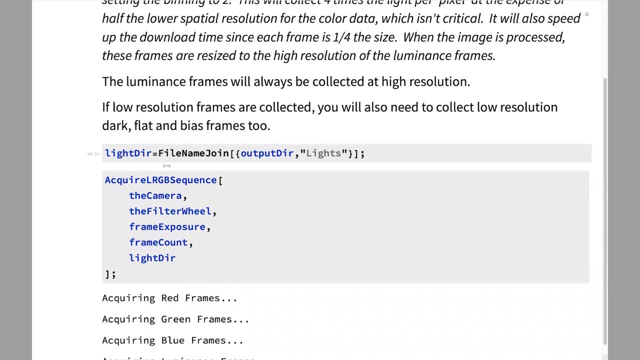 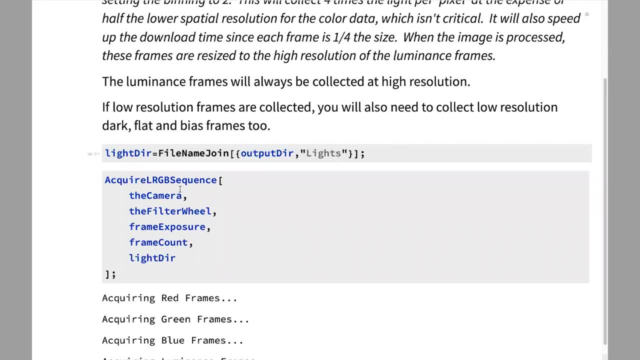 And take frame count exposures for each one of them at frame exposure, And it will store them in that directory, And so you may have 20 exposures on each one of them. But you don't have to do anything Because it's all automated by that function. 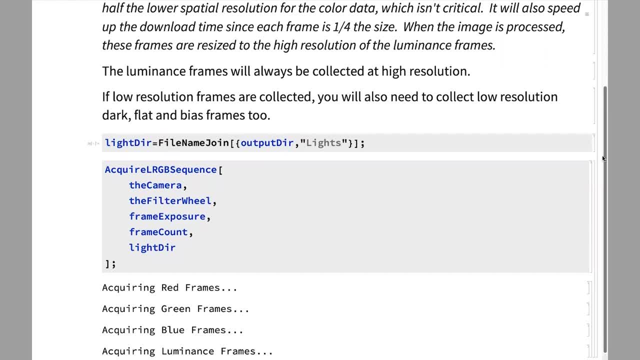 And the source for that function is in the astro device package. So it will acquire red, green, blue and luminance frames And you can go inside, You can make hot chocolate, You can watch something on Netflix And just let the camera munch away. 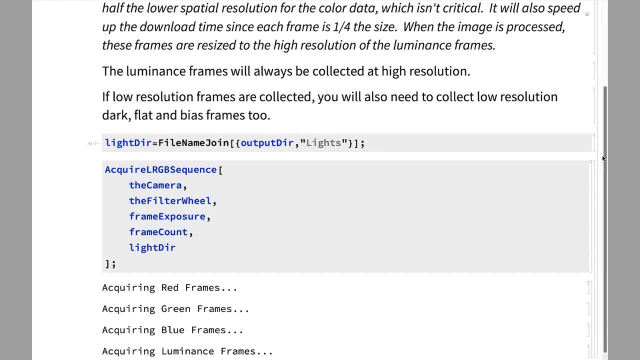 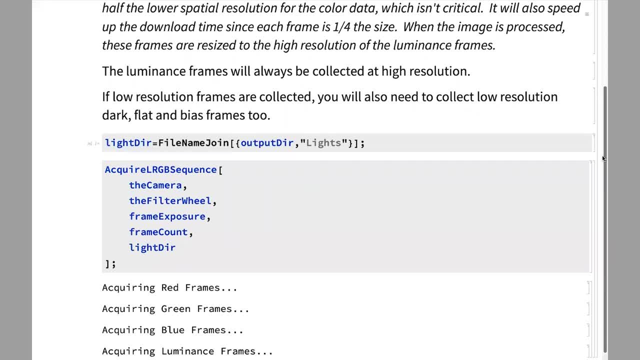 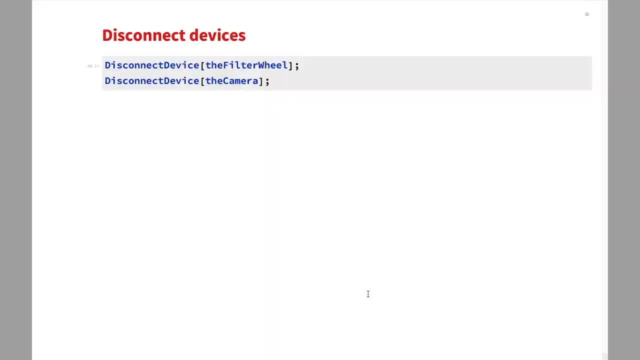 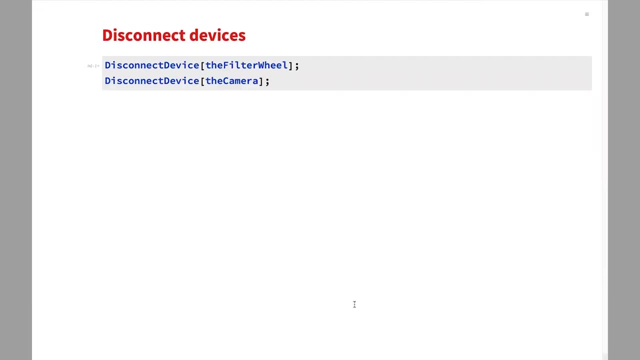 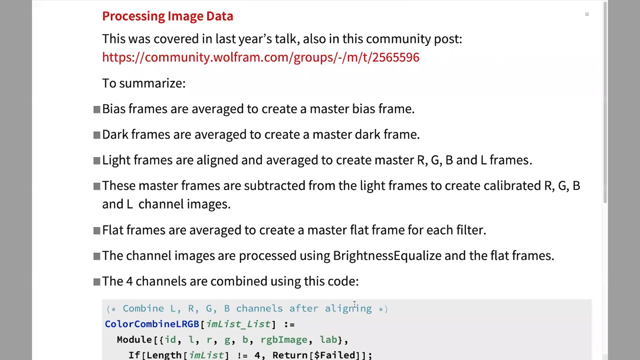 So at that point you just need to do the processing Now. I talked about the processing procedures last year at the talk, So I'm just going to kind of gloss over them a little bit, And I've also covered them in a community talk which is listed up there. 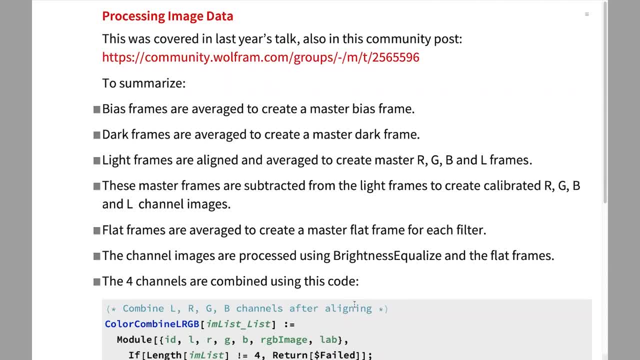 And that goes into more detail about how to create the final image, but i'm just going to go over it briefly here. so for the bias frames, you average them to create a master bias frame. same for the dark frames: you average them to create a master dark frame. and then the light frames are lined and averaged to create master red, green, blue and 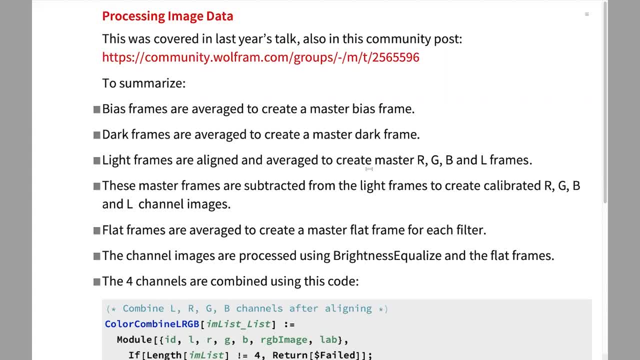 luminance frames, and those are with the technique used in this community post and also from last year. the actual details of the alignment algorithm are actually in python, so this shows you another strength of Mathematica that you can use it to call out to different languages, as it turns out. 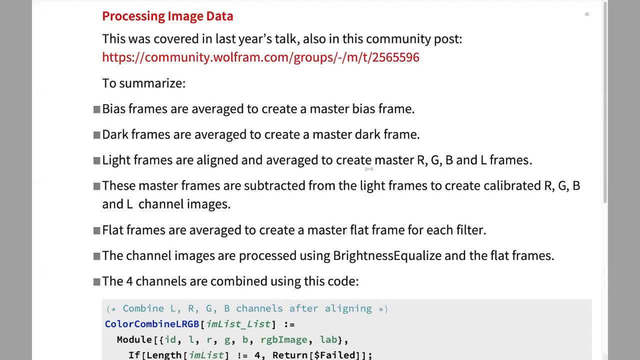 there's some very good routines for aligning stars fields in python and we don't have to translate that into the wolfram language, we just call those routines and so, and you can actually put the python code right into your notebook and that's all detailed in that posting. so that's how, uh, light frames are aligned and averaged to create. 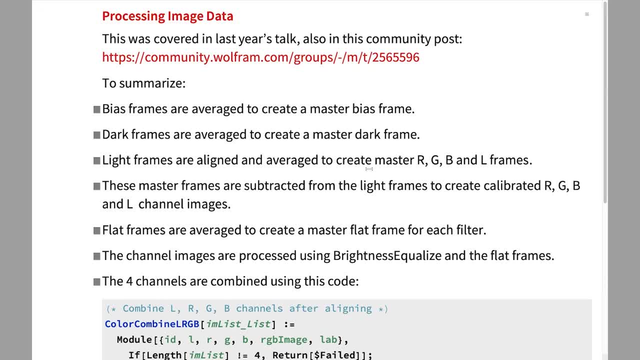 the master, uh, uh, color channels. and then, um, you take, you subtract out the bias, the dark uh frame, uh, noise and um, that will create calibrated frames. and then, uh, you process your flat frames, which is just averaging for each one of the channels, um, and then the channel images. 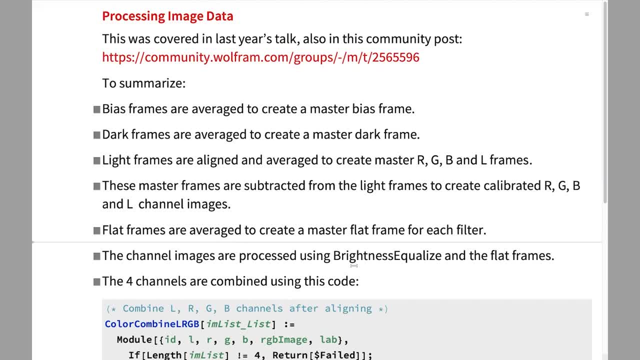 are processed using another, uh, wolfram language, uh, feature brightness equalize, which will spread brightness and subtract out things like dust modes, and that will take a flat frame and the harbor for a flat frame you want to equalize and it will produce a final frame and then the four. 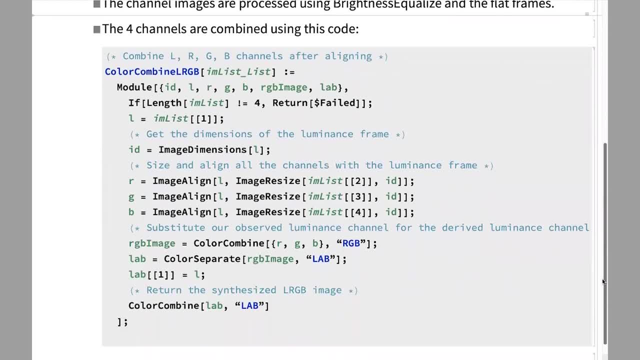 channels can be combined using this code, which is also detailed in that posting. so this is color combined: l, r, gb, not uh, it's not just three channels or combining four channels. i'll just describe briefly what this is doing, um, so it does some checking. the first channel is: 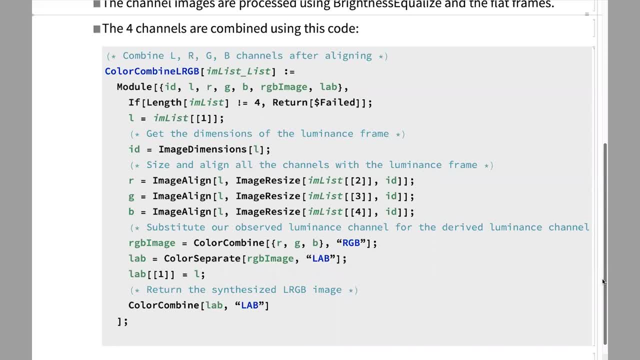 assumed in the list that's passed into. this is assumed to be the luminance one, so it gets dimensions of the luminance channel and then it, if needed, it resizes the color data to fit the luminance data and then it lines it using image align. i don't need to use the python routine for. 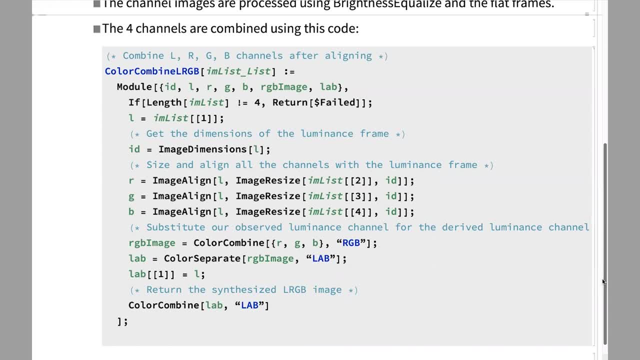 this because at this point the images are pretty bright because they've been stacked up and our normal image line works pretty good for that. and then i combine just the color channels to get an rgb channel, an rgb image, and then i convert that to an lab image, which is an image that has three 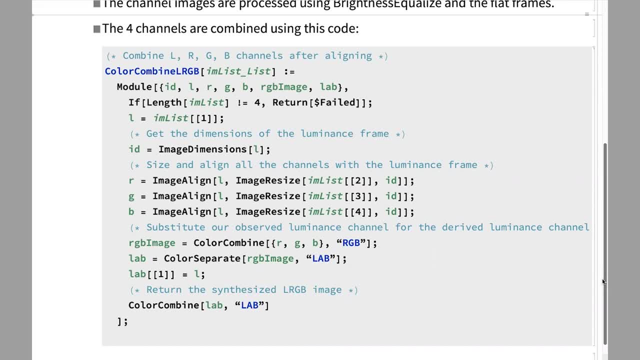 channels, two color channels represented by a and b, a luminance image, and then i take out the luminance and i plug in the luminance that came from our direct observation and then i recombine it in the lab color space and that will produce the final uh lrgb image. 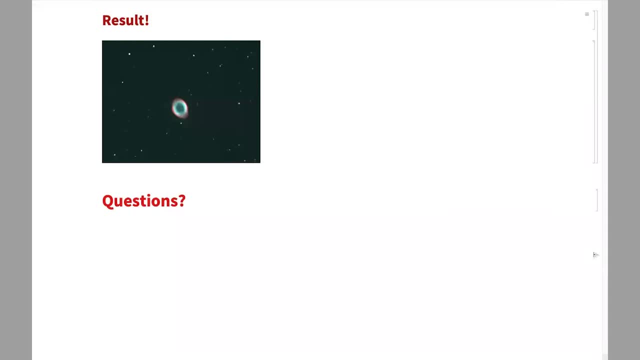 so, and there it is. so that's, uh, the ring nebula produced in this manner. so so that's it. any questions? uh й, well, yeah, it has to be focused on infinity, otherwise you're going to get artifacts of the, the telescope, in on the flat frame, which which you don't, which i've done before. but you don't want to like if an optimism is a trick or a strategy. once you start using the zero scientist, out of a classical apocalypse, you're going to get artifacts of the, the telescope, on the, the platform, which you don't, which i've done before but you don't want like if i did it for impulse. you're going to get this here, this beautiful ridge, if the telescope 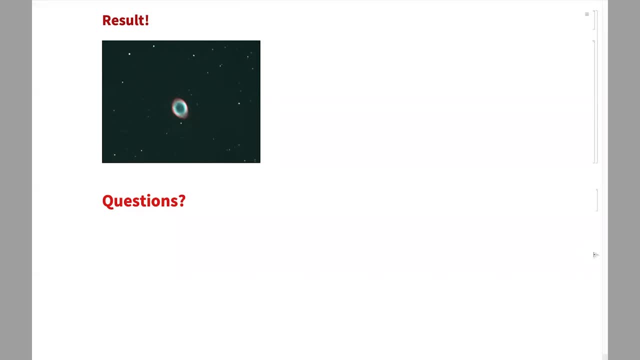 you have a Schmidt-Cassegrain scope, you're going to see kind of a donut-shaped thing which is because there's an obstructed optical path. So yeah, same focus, put a t-shirt which helps distribute it more evenly, and that works great. So yes, sir, I have an idea of using a. 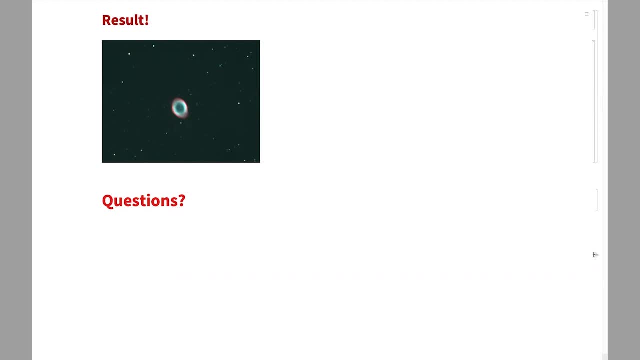 James Webb telescope and images. You can absolutely do that. There's a website set up and I've been on this website and the data is humongous, as you might guess. but you can download every single image taken by the James Webb Space Telescope and not just the final pretty color images. You can. 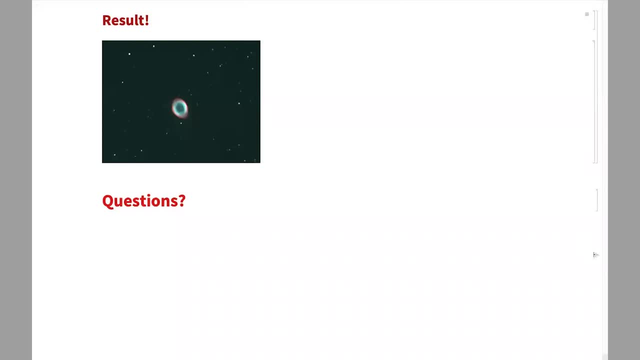 download these subframes and process it using exactly this technique and you can create your own images, and a lot of amateurs have done that. They've seen if they can improve on the James Webb and the NASA processing. So, yes, I encourage you to do that. The images obviously are very high. 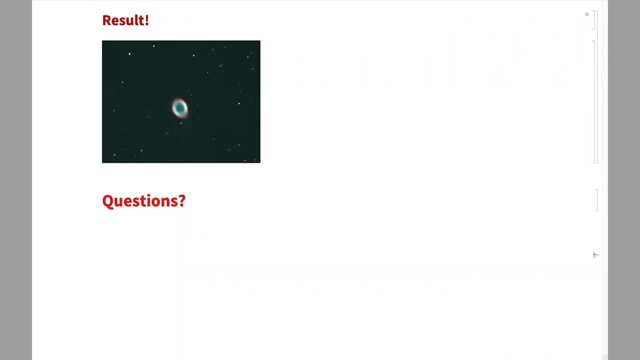 resolution, but it's a good, rewarding thing to get into astrophotography using the best telescope we have available. What is that site, or what can we search for to get to that site? Oh boy, I'll have to send that to you. I've got it on my other computer, but yeah, and it's a little. 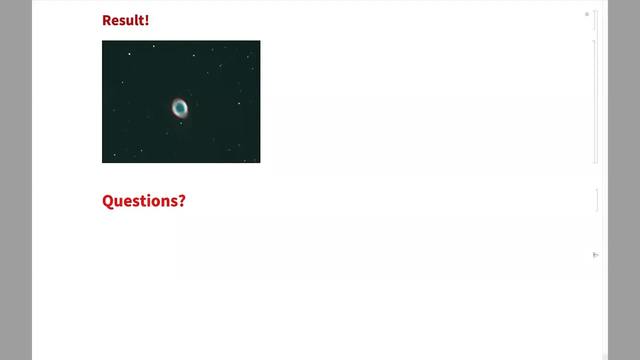 bit tricky to find. It's a little bit tricky to find what you want because the stuff- there's a lot of stuff in there, but all the observations are all listed in there and all the data is in there. So, and they're all FITS files which this works with. Yes, sir. 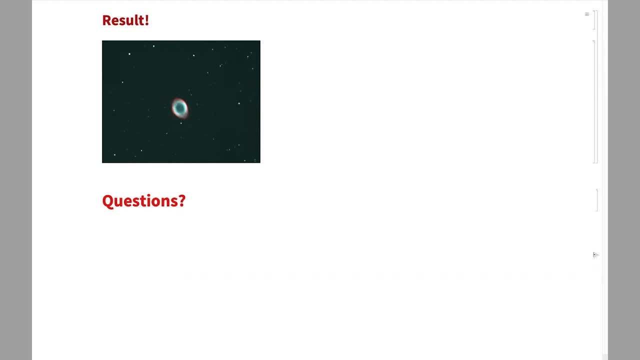 Would the current package run using the other? I saw the NET, so it's running. the other folks Probably will work that way too. Yeah, I haven't tried that, but it's probably, yes, probably. yes, I had forgotten about that. 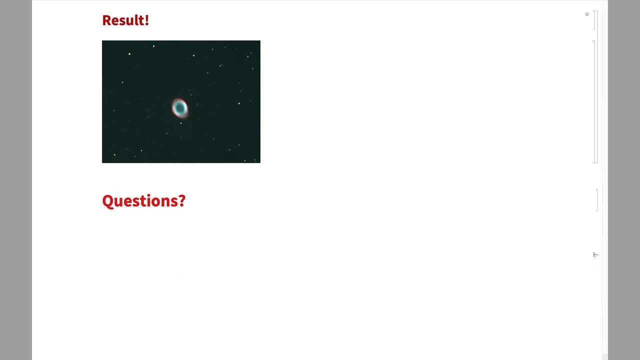 Let's see how are we doing here on time. Have you talked about putting it in the package repository? Yes, I was going to. I was trying to do that yesterday and then I thought I'll just ask Jeff. I'll just ask Jeff, He'll help me do it. So the second best thing: I just included it with the talk. but there's other stuff in the, in our little. 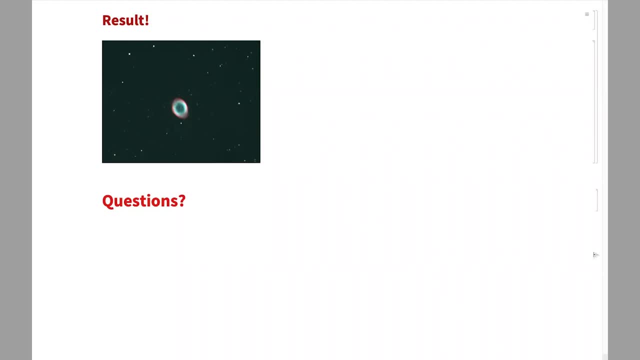 collection which Jeff has contributed to. it's not just me that we should put the whole, the whole thing, in the package repository so anyone can use. and it's not just this sort of stuff, it's like image processing stuff and alignment stuff and photometry stuff. 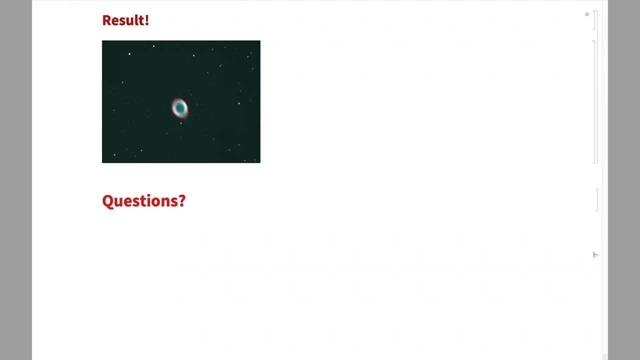 So it's all. it's all good stuff and we're going to publish it all, but for right now, you got the stuff that talks to ASCOM. Well, I mean, images are images, and if you're telescoping, 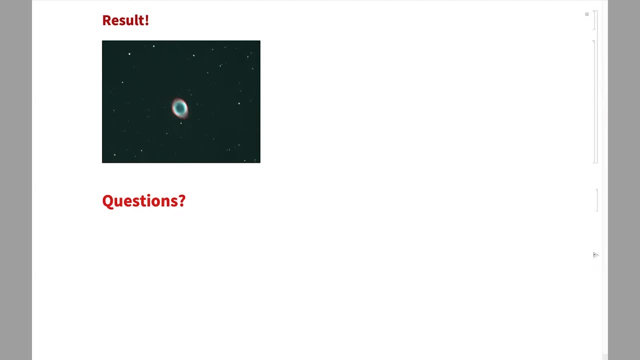 if the telescope is is locked on to an object, it will stay there pretty good. I mean, Oh yes, that that's also a possibility, but remember, the main thing that would drift would be the temperature of the camera and since the camera is is a closed loop type of thing, it's being refrigerated at a specific temperature. 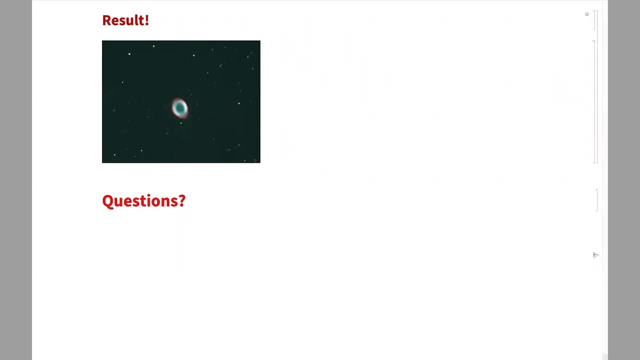 That's why you can build a library of like dark frames. So that's so. if you're in the in you're shopping for an astronomical camera, make sure you get something that you can. it's regulated. you can set to a certain temperature. most of them are nowadays, but that's okay. so I think, okay good. 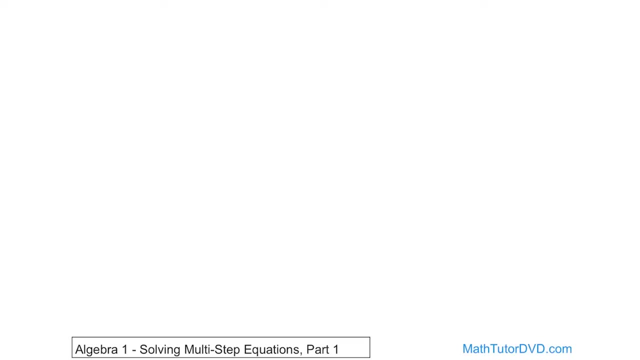 Hello, welcome back to Algebra 1.. Here we're going to solve what we're going to call multi-step equations, And it's a really important concept. So what we've learned before is how to solve single-step equations, where all you had to do was add or subtract, or all you had to. 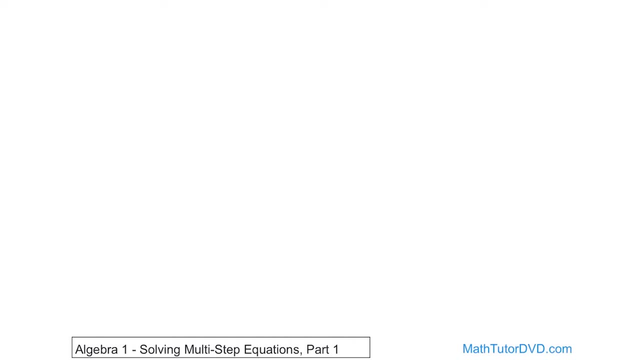 do was multiply or divide to get the answer. And now we're going to have some equations where you may have to do both: You may have to add and then divide, or you may have to subtract and then multiply, or something like that. And they're not hard, it's just we're. 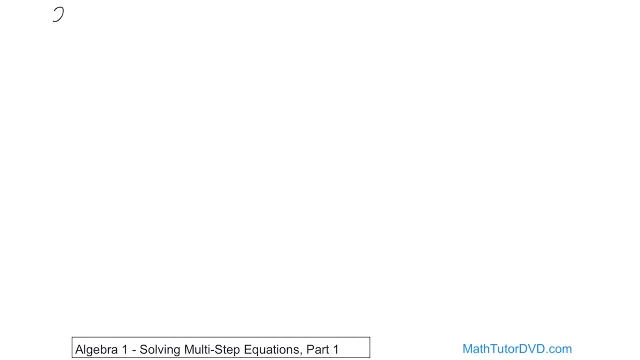 building on the skills that we've learned before. So, for instance, if you have the equation 2x minus 1 is equal to 11.. Now this one's a little bit different than what we've seen before, because notice that we have multiplication going on here, but we also have some subtraction. 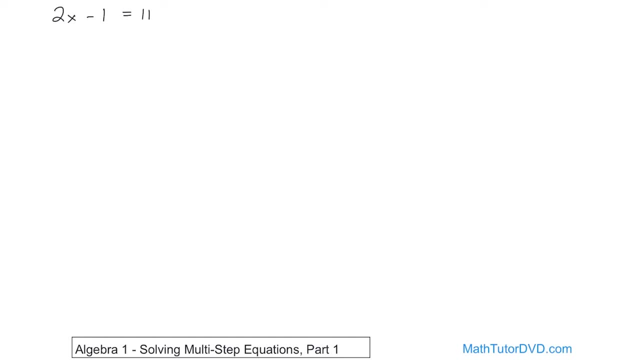 But the goal is the same as it is in all of the other lessons. We want to get x by himself And you have to view this as a puzzle or maybe a Christmas present. You have to unwrap it And, even though you really want to get to x- really, really bad- and get the answer,